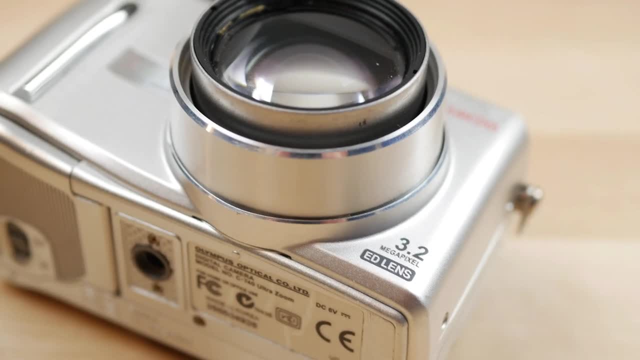 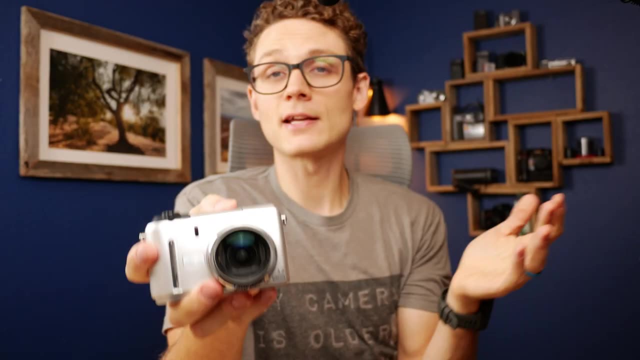 a little awkward in the pocket, too big for that, and i chose it for this experiment for three reasons. first, it's cheap. you can grab it for under 10 bucks on ebay any day of the week. second, ally covered this camera in great detail on her channel. one month, two cameras. 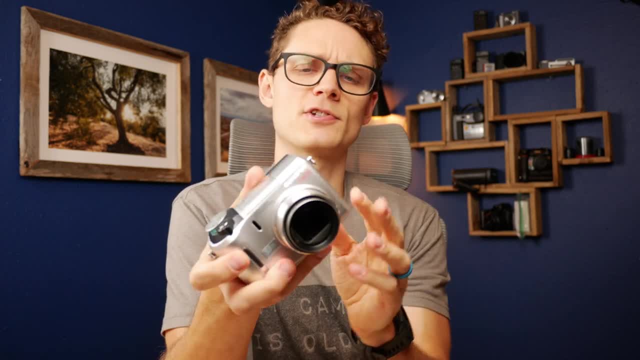 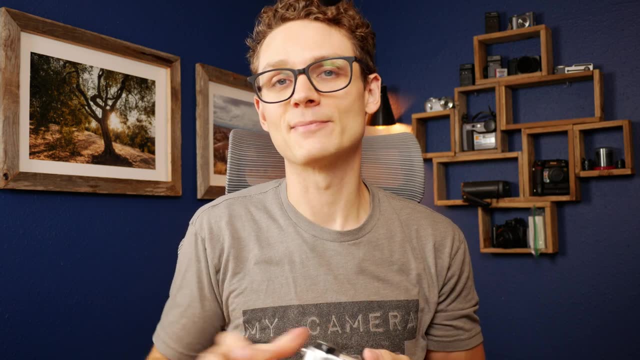 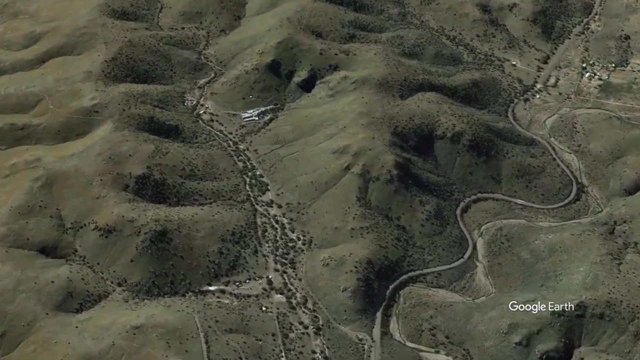 and, uh, really loved what she got out of it for such a cheap little camera. my first olympus point shoot, so that was interesting. and then, third, and the real reason i chose this camera is because of this, but we'll talk more about that later. my first opportunity to photograph with this camera came after we set up camp and went on a. 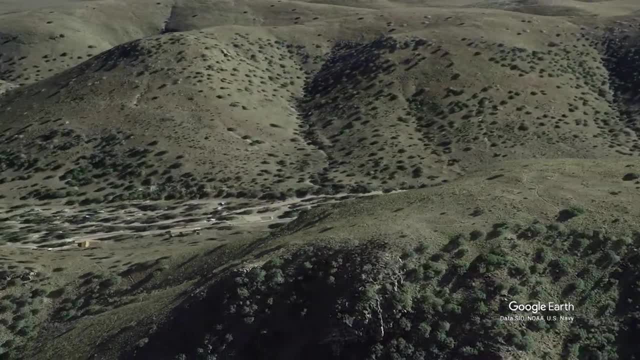 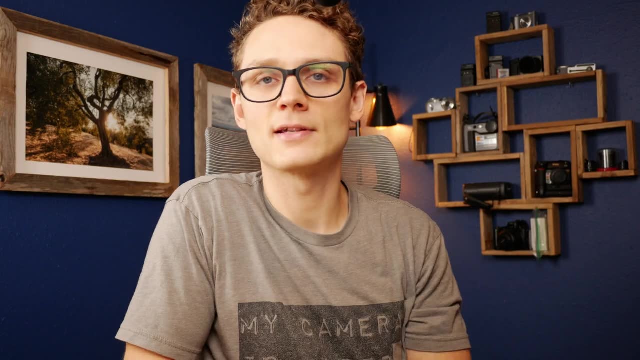 short hike in davis mountain state park here in texas. they call it a mountain. here in texas we don't have a lot to go off of, so it's not very big, but i guess it's technically a mountain. in any case it was beautiful out there. i loved it in that state park when we went on the hike. 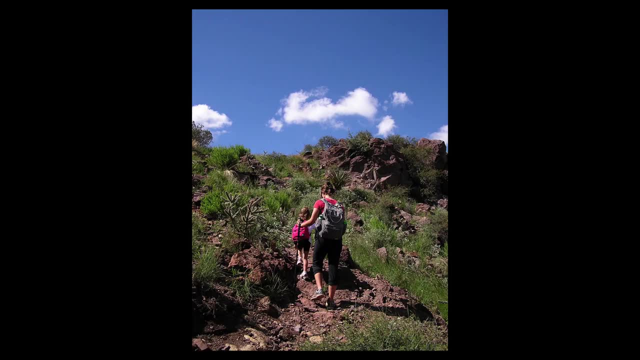 out there. i loved it in that state park when we went on the hike out there. i loved it in that state park when we went on the hike. the sun was high in the sky, but the kids were cheerful and that is what determines when and where we go on a hike, not silly stuff like perfect lighting, but i was still impressed. 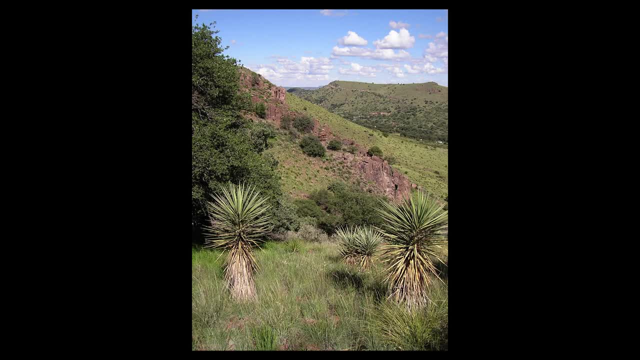 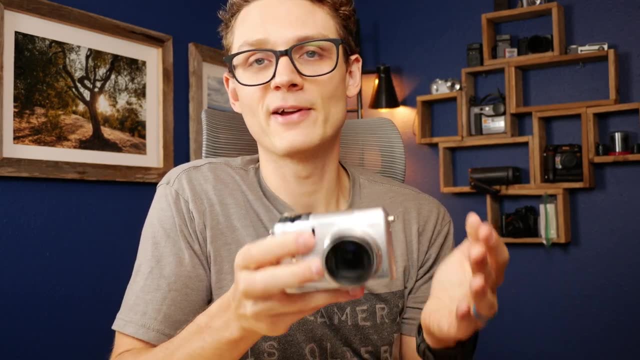 with this little camera could do. now the camera by default over sharpens your files like crazy. at first i was looking through the images on the playback thinking, wow, that's super impressive. this lens is super sharp. until i pull it up on my computer and realized that it was. 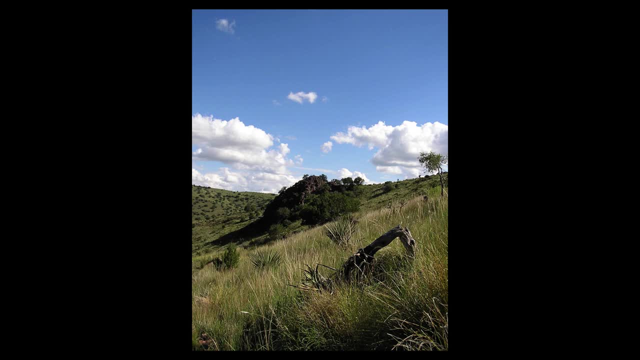 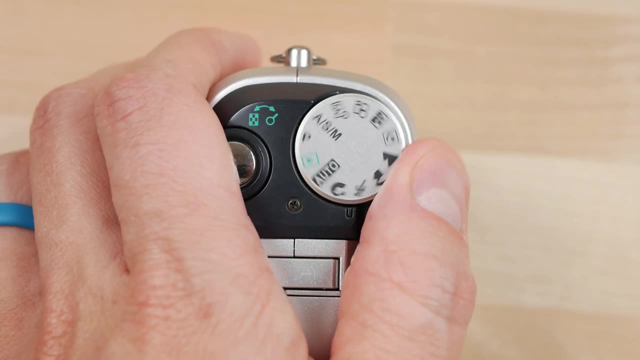 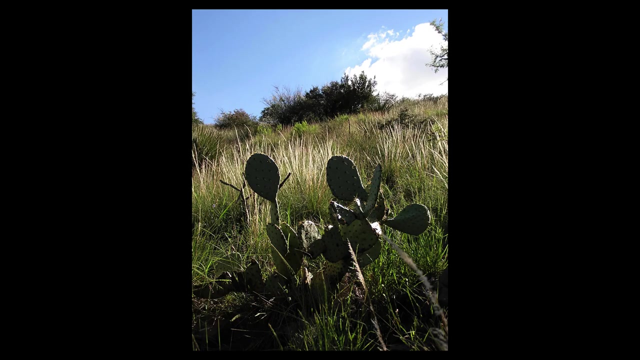 way too sharp. a lot of these pictures are left on that default setting, so that's what you're seeing. it was only later that i learned the hack that ally talks about in her her video, where you set up your own profile and then save that setting each time you reboot to a lower sharpening level. 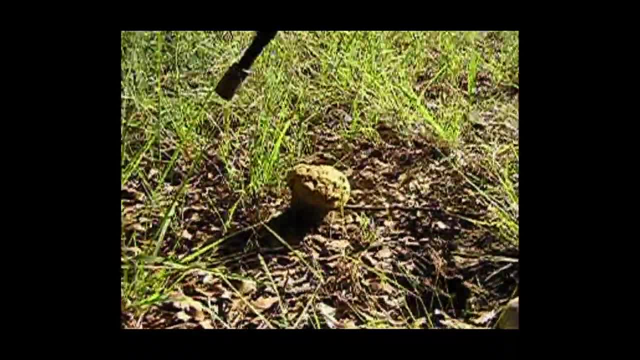 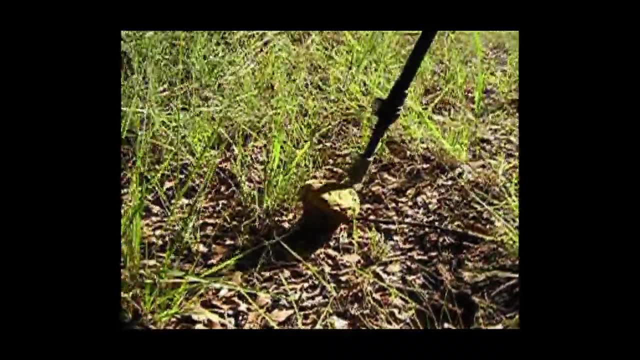 it was also on this hike that we discovered this green smoke emitting mushroom and that this camera can shoot video. i don't know which is more shocking. seriously, if you know what this is, let me know. as part of this trip, we plan to visit balamaria state park, which is this: 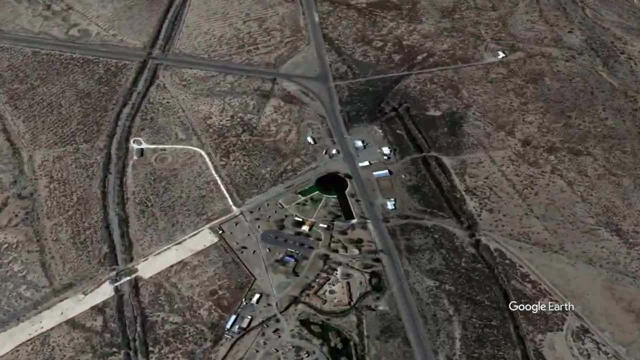 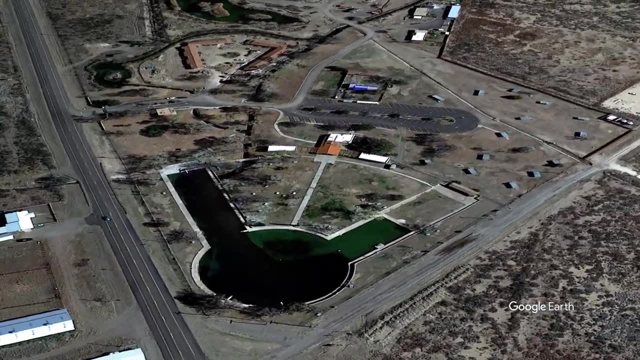 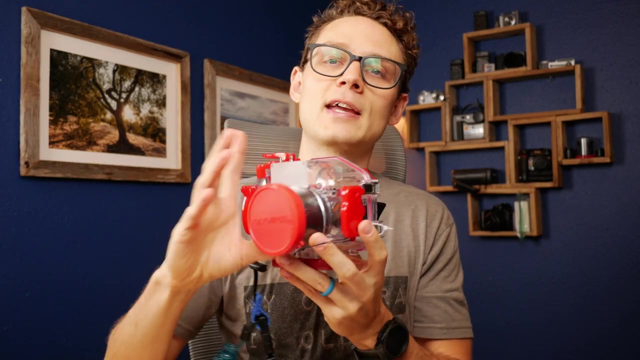 spring-fed swimming hole, literally an oasis in the middle of the desert, this amazing clear water pool that people uh snorkel and you can see fish and turtles down there. unfortunately, because of recent rains, the water was murky, so i didn't even get to bust out my cool underwater case that i bought for this camera. 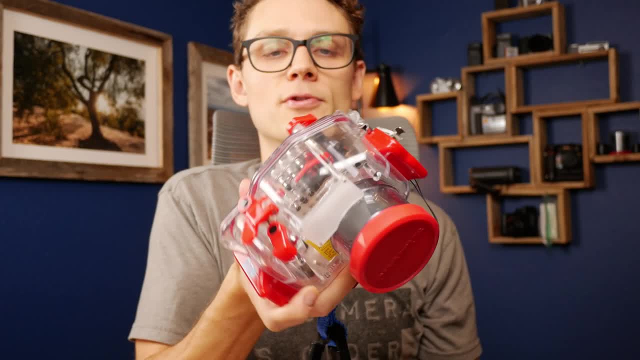 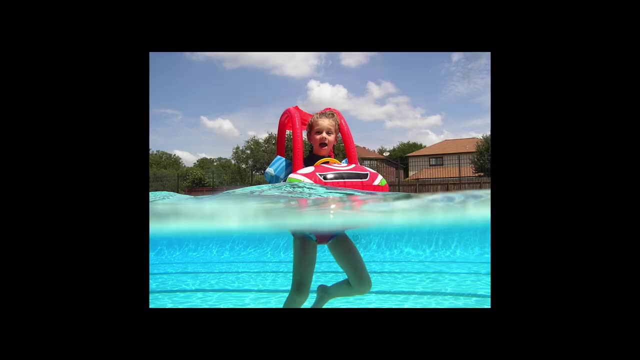 so this just sat up and took up a big portion of my little toyota corolla for the whole trip. but i just wanted to test it out again. i've never done it in my life, so i'm so excited to test it out. so we get to test it in a pool, our neighborhood pool, a couple weeks prior, and the results are: 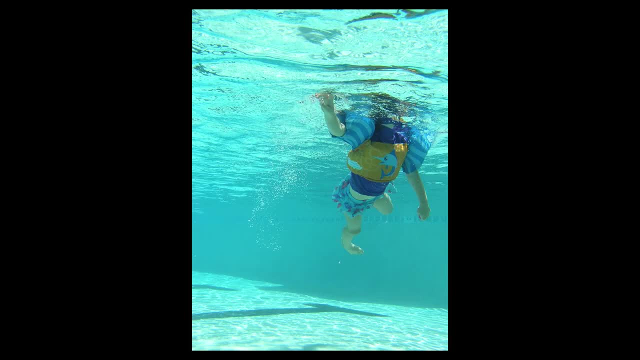 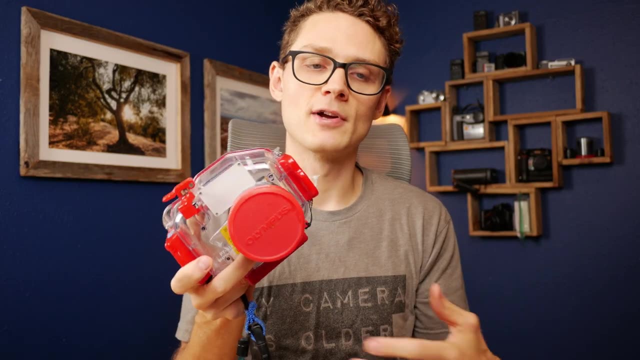 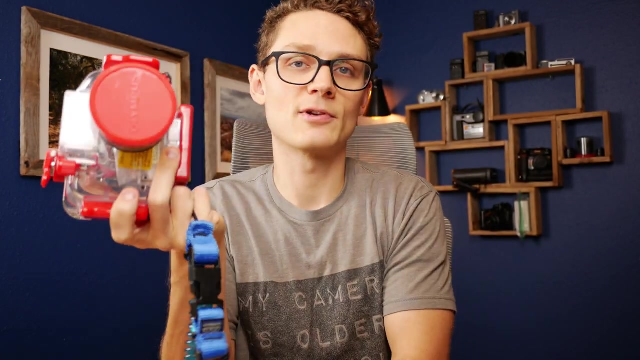 promising. it's kind of a dream of mine. ever since i was a little kid looking at these dive cases, i always wanted to own one, but they're always so expensive and the cameras are expensive too. nowadays you can buy one of these old cameras for five bucks and one of these cases for 20 bucks- any. 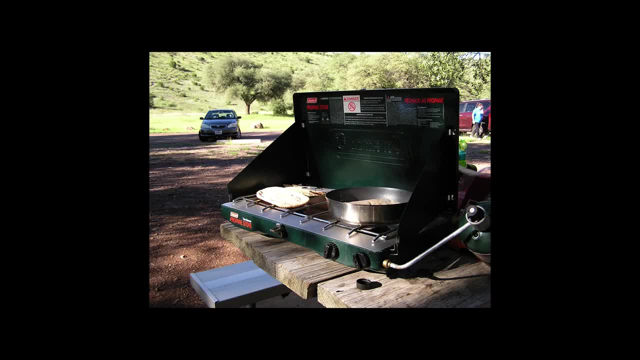 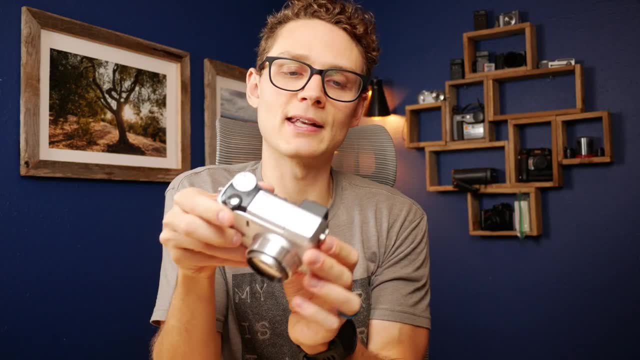 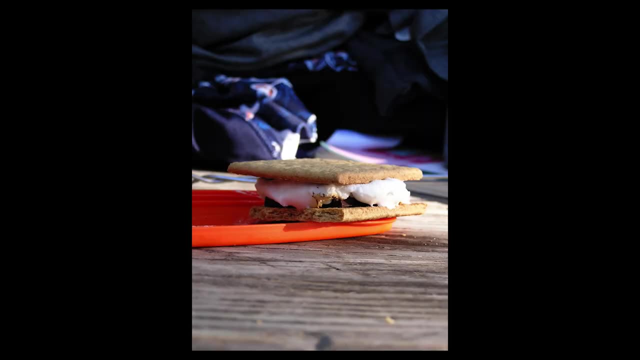 day, so i think that's pretty cool. I whipped out this Olympus to try my hand at some food photography and while there's nothing award winning here, I appreciate this cheap little camera's lifelike colors and rendering. It was here. I played more with the macro mode on the camera and got some real bokeh Shout out to. 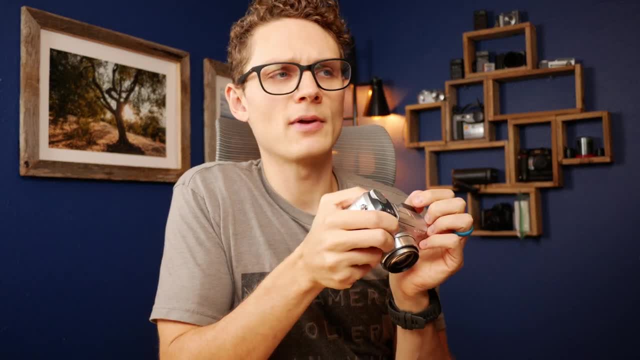 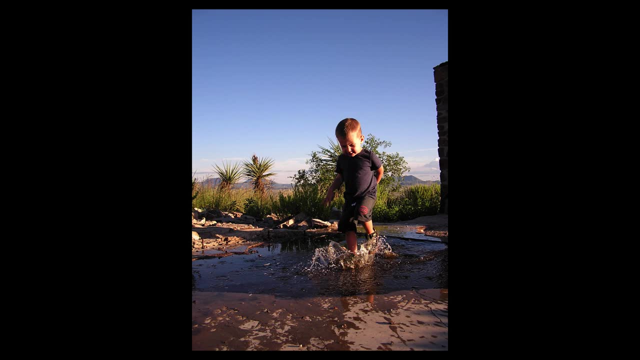 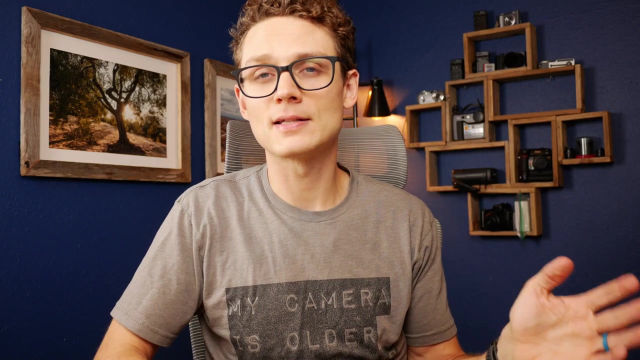 s'mores, by the way, as being one of the best parts of camping. and my question to those who are not from the United States: do you even know about s'mores? Is that a thing around the world? I don't know. Sunset was approaching fast and we wanted to see the sunset and see how this camera performed. 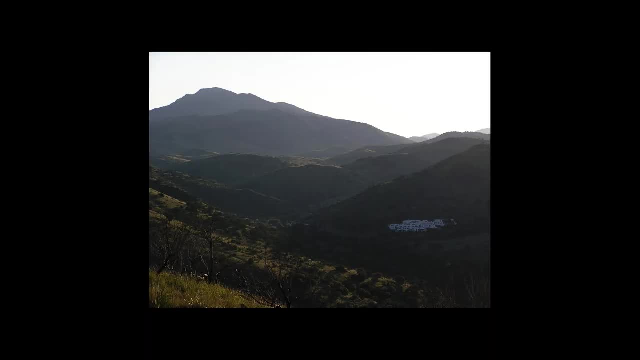 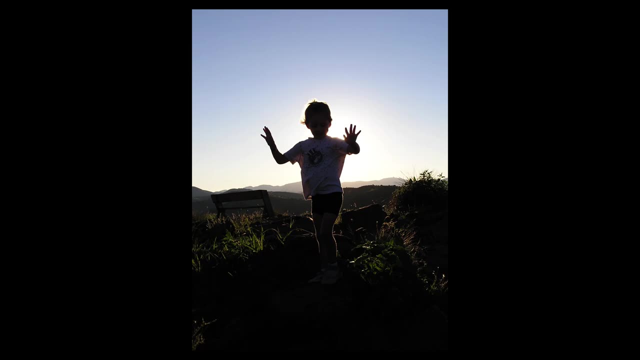 in that nice light. so we drove up to this little overlook And incredibly, this lens doesn't show any horrible chromatic aberrations to my eye. Even if you look at it from a distance, it's not that bad. Even if you look at it from a distance, it's not that bad. 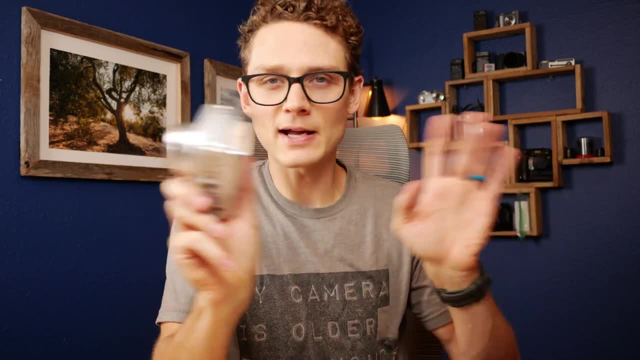 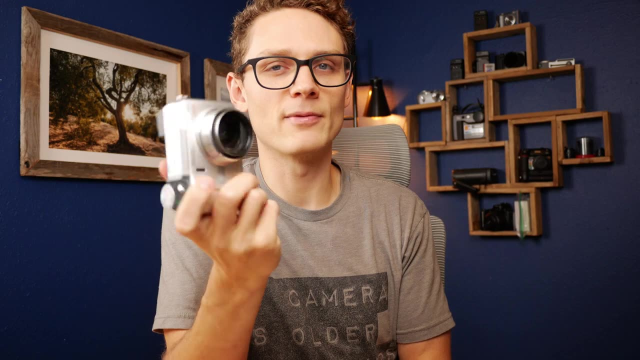 Even if you look at it from a distance, it's not that bad, Even in this extreme backlit scenario. So I take back any comments I made about the over sharpening and trying to make up for a lackluster lens here. I'm actually really impressed with this lens at this point. 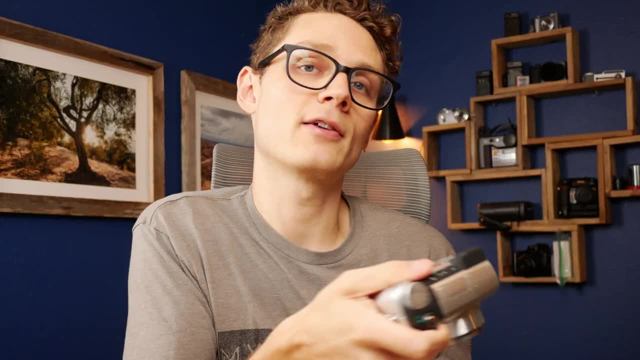 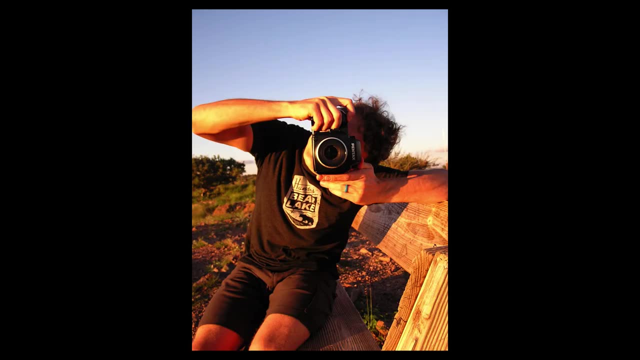 And because I wanted to try out another camera that I brought- because, you know me, I don't just bring one camera on a trip. I handed this camera off to my four-year-old and let her have at it, And that's when I found out she was a better photographer than I am. 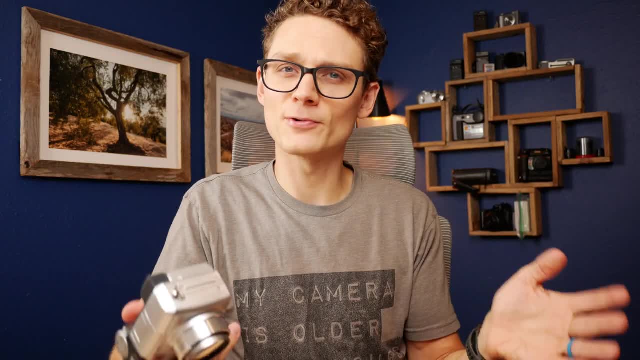 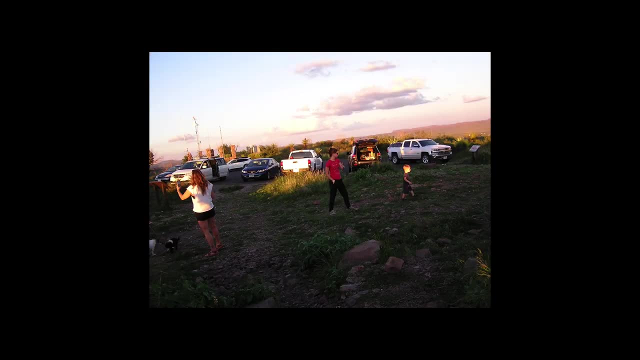 I mean she had a few Star Wars reboots in there, but overall some really cool stuff. And, in all seriousness, if all you get out of this video is to buy a $5 old digicam and then hand it to a young person in your life, then my job here is complete. 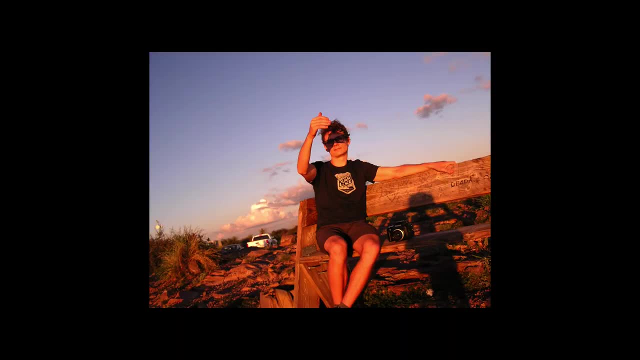 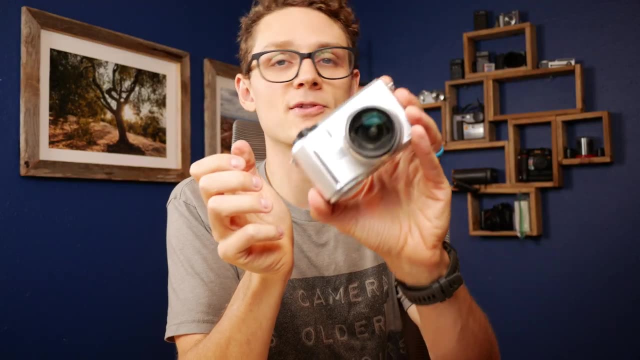 It is fascinating to see what their little minds visualize And grab ahold on it and then are able to take a picture of. And then, unlike this little guy stealing my expensive wildlife camera setup, these cameras are much more inexpensive and if they break it, that's fine. 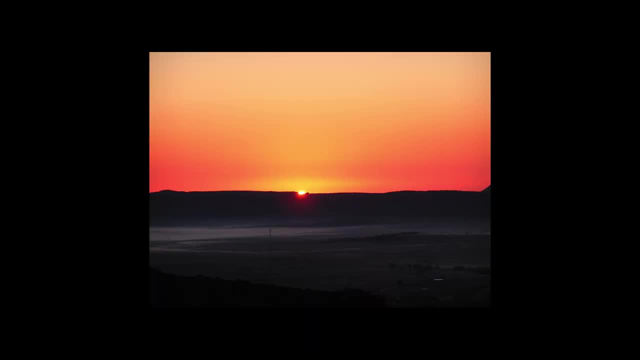 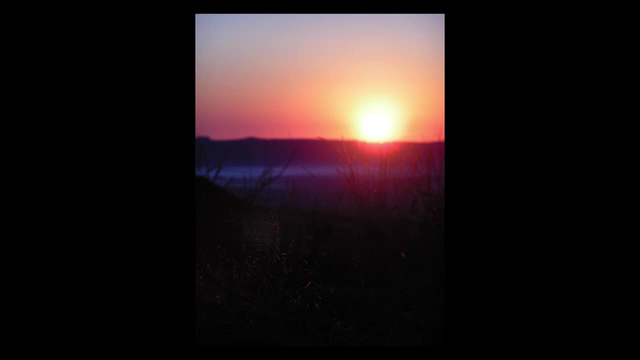 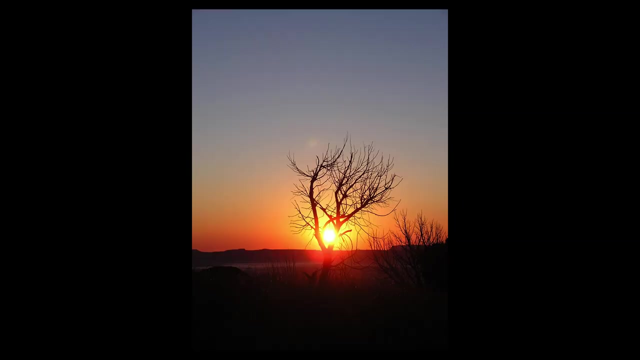 We woke up early the next morning with surprisingly compliant kids to go catch the sunrise on that same overlook, And the camera had a little difficulty focusing in low light and backlit scenarios. but even some of these out of focus shots are really smooth and pleasant. 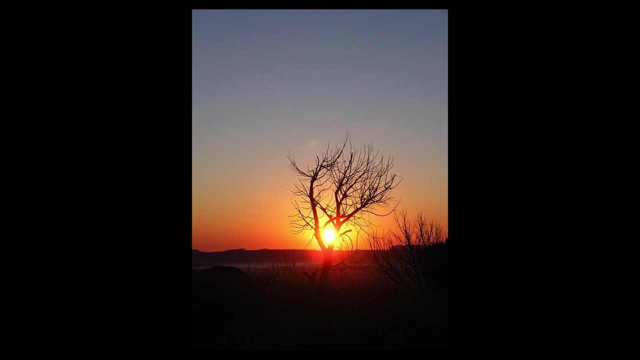 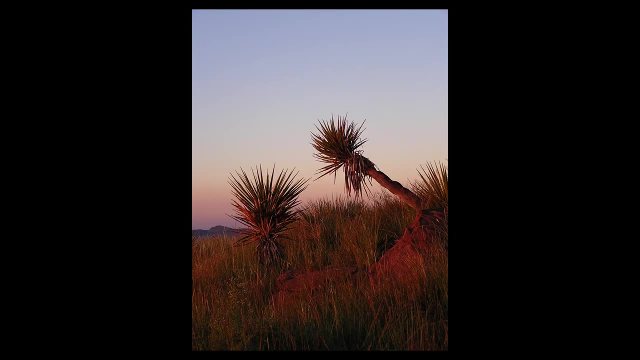 And I'm slowly learning, thanks to some other photographers who have influenced me, that we shouldn't really overly focus on the technical details of photographs. If we're trying to convey a mood or just some creative expression, then it's okay to break some of those rules. 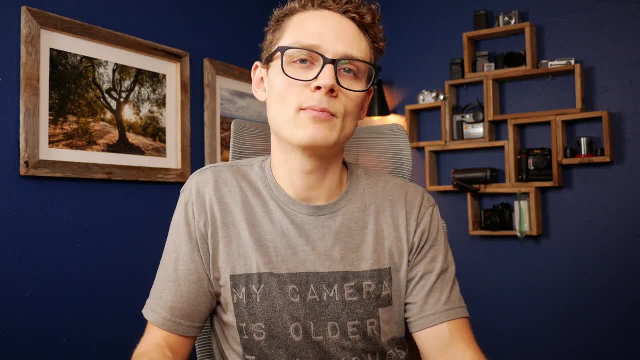 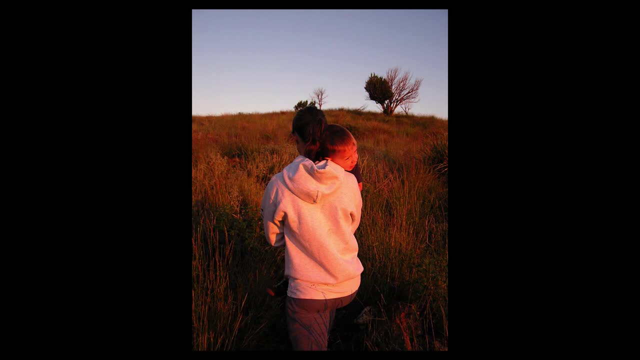 I'm just saying maybe you shouldn't just avoid all that altogether, but maybe embrace the beauty of the sun and see where that takes you. And then it was on our way back to the car from this little walk down the overlook that I got some of my favorite pictures from the trip. 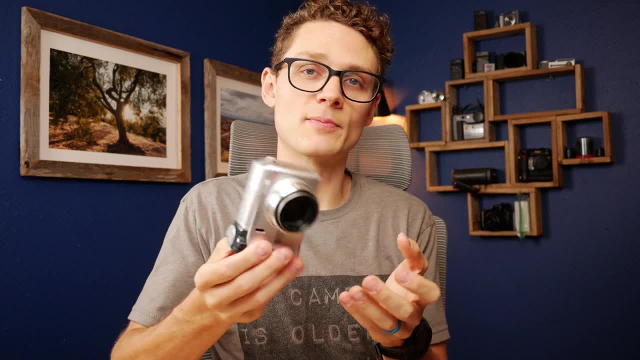 The light was just beautiful coming off of the sunrise And once again, I think the Olympus just nailed the colors straight out of the camera for these, And it was at this point I was feeling pretty good about this little camera and what I was able to get so far. 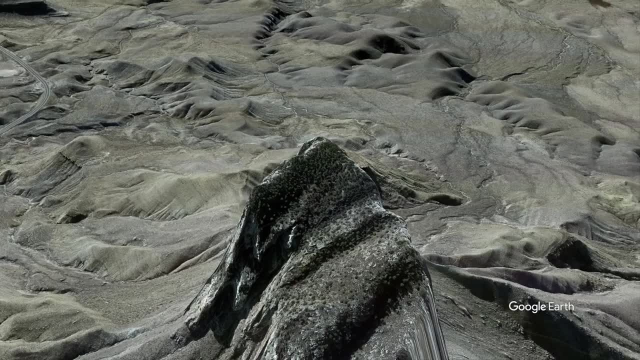 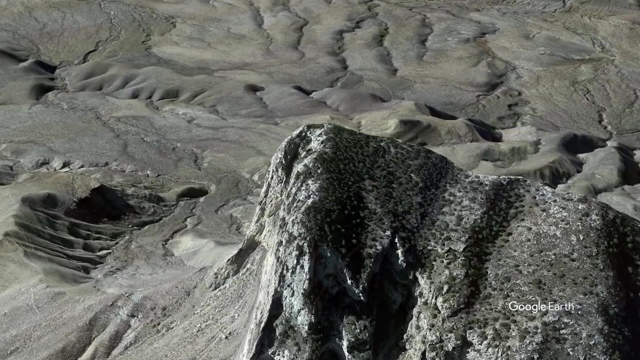 But little did I know that some of my favorite shots were yet to come From Davis Mountain State Park. we then drove to Guadalupe Mountain's national park To camp there for a few nights, And my kids were understandably worn out from two nights of camping and me taking them on hikes. 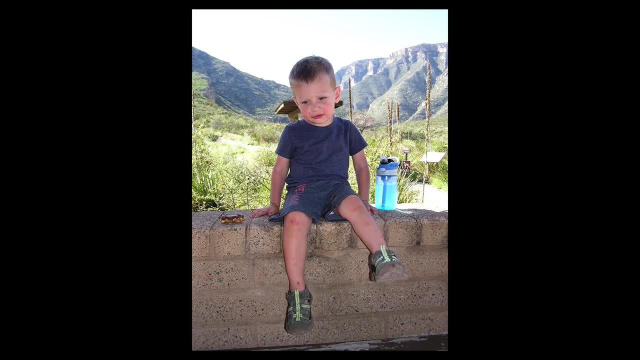 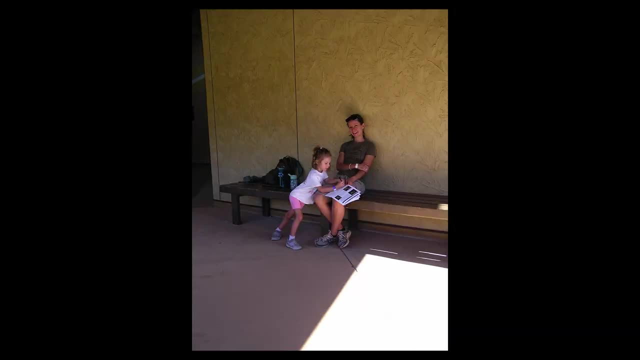 So they didn't want to hike anymore. That was the inspiration for this picture. I call it. are we there yet? It was a good chance to try out the flash on the Olympus C740, which turns out is pretty good. I feel like it balanced the scene well. 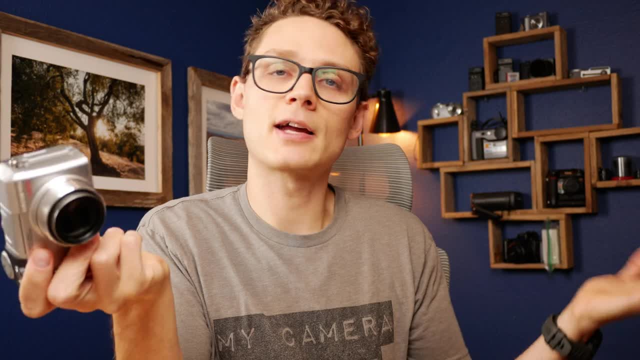 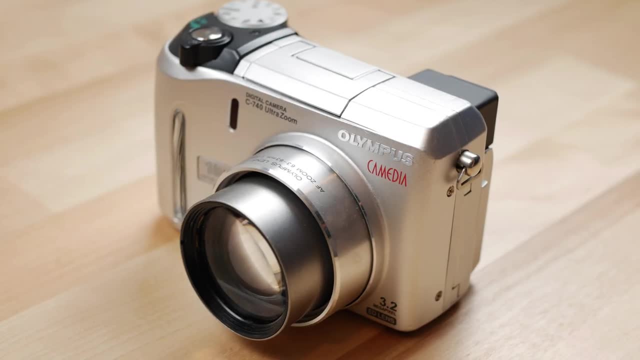 And while it definitely looks like the picture was taken 20 years ago, I kind of like that vibe And I almost forgot. this camera is called an ultra zoom for a reason. It has a humongous zoom range: 38mm To 380mm, equivalent on the long end. 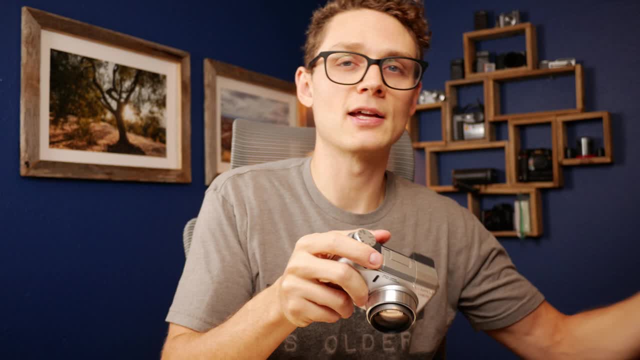 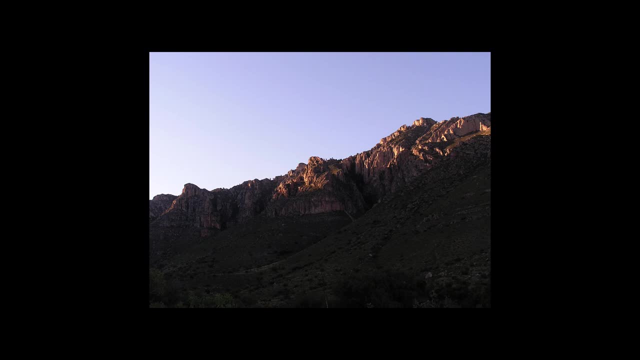 I would say that the optical quality degrades quite a bit on the very long end And certainly it's hard to stabilize a camera that doesn't have any stabilization. But back off the zoom range a little bit and I'd say it captures plenty of detail.